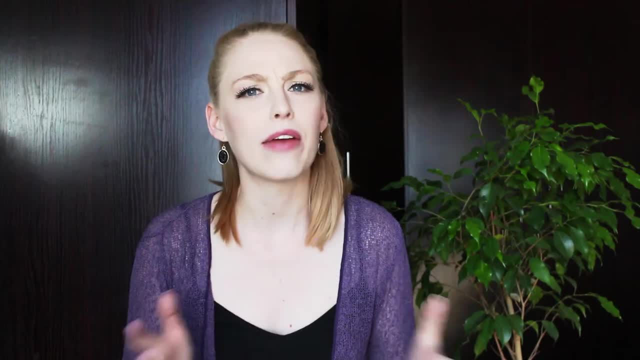 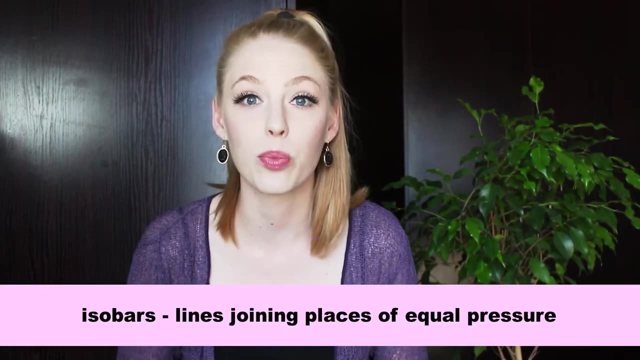 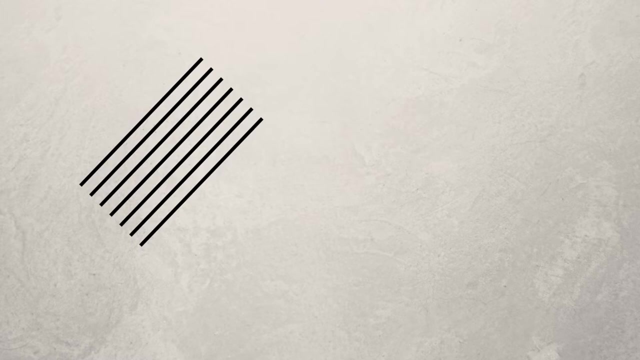 force is and the stronger the wind will be. If we are looking on a weather map or on a synoptic chart, we can use our isobars, which are lines joining places of equal pressure, to help us determine what the pressure gradient force will be If the isobars are closer together. 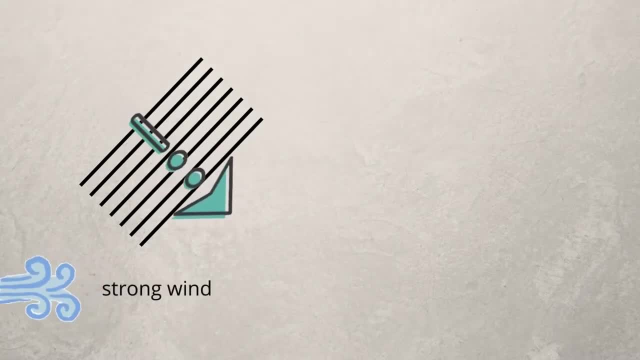 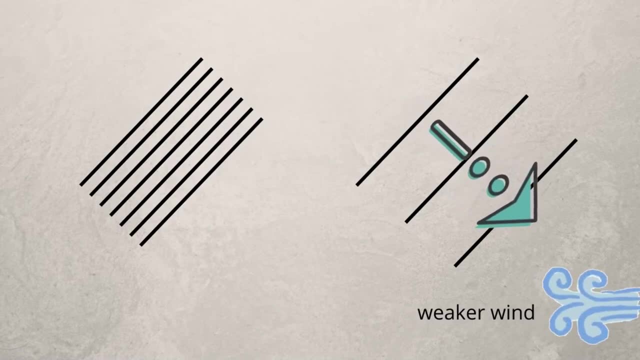 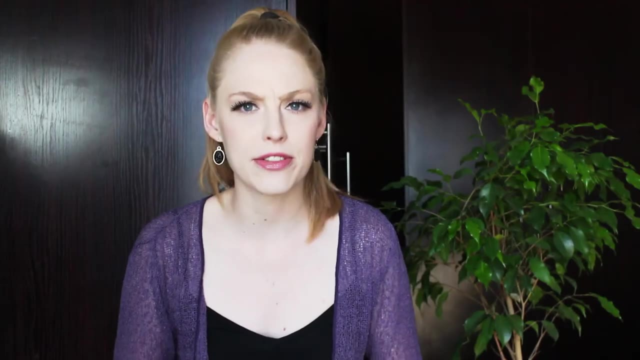 we say that the pressure gradient force is steeper and therefore the wind is stronger. If the isobars are further apart, it means that the wind will be weaker. The next concept that plays a major role in the movement of air around our globe is Coriolis force. Coriolis- 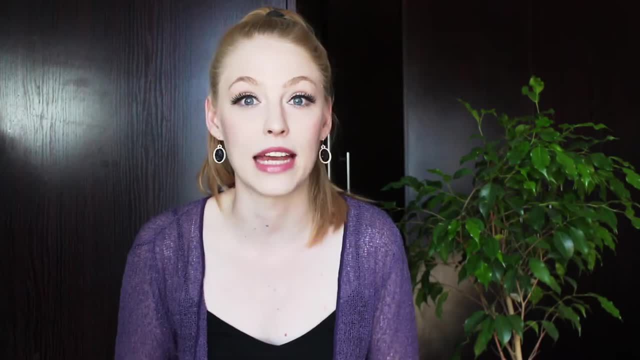 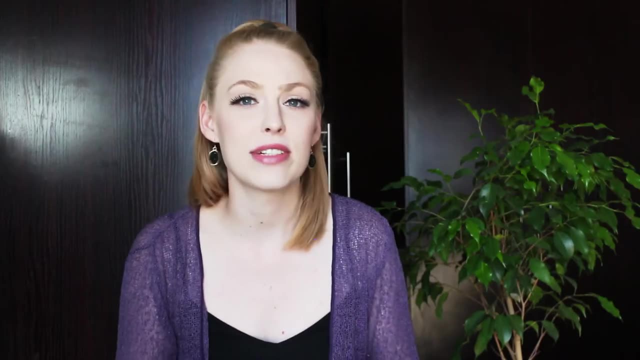 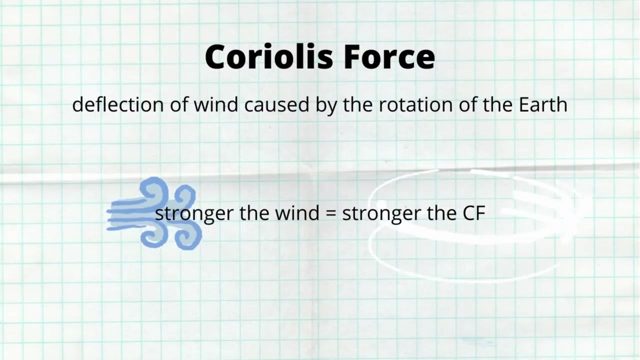 force is the deflection of wind that is caused by the rotation of the earth. Coriolis force is at the poles and weakest at the equator. In fact, there is actually no Coriolis force. five degrees north and south of the equator, The stronger the wind is, the stronger the 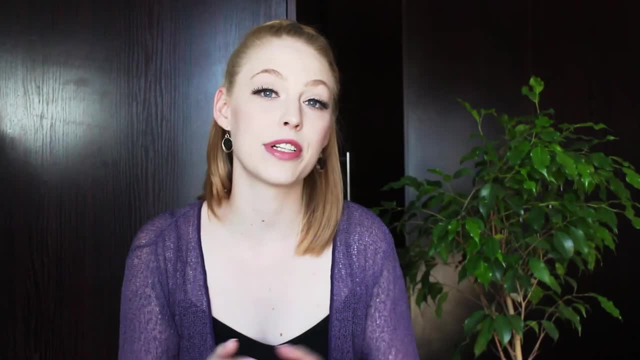 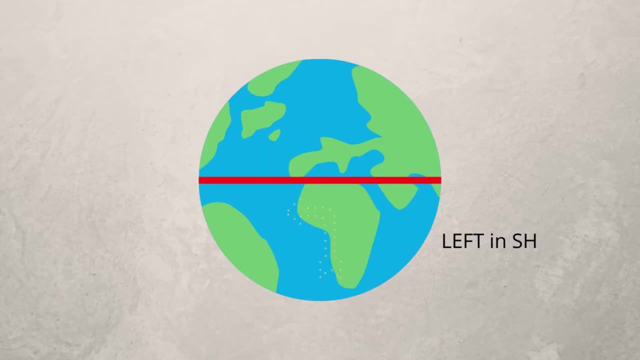 Coriolis force will be. Now, winds deflect in different directions depending on what hemisphere we are in. In the southern hemisphere, winds deflect to the left, and in the northern hemisphere, winds deflect to the right. This rule is known as Farrell's law. A third concept. 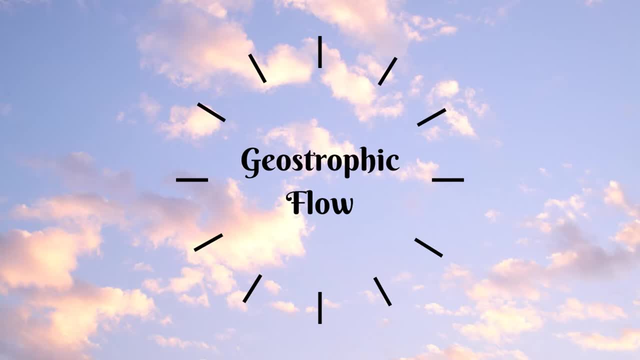 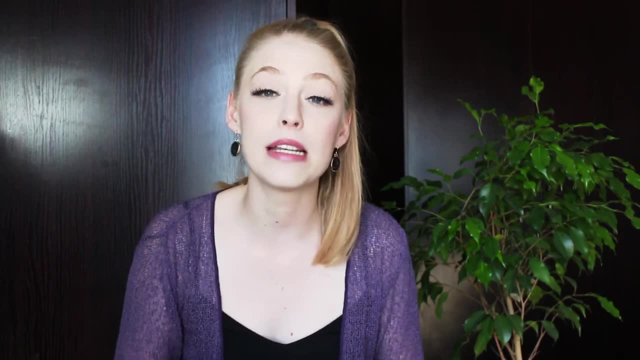 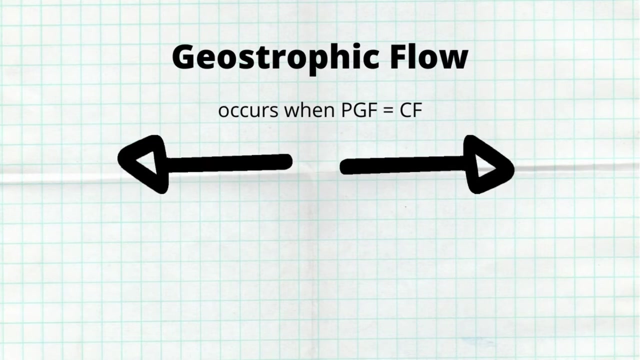 in mind is something called geostrophic flow. Now, geostrophic flow occurs when wind actually blows parallel to isobars. In other words, it is perpendicular to the pressure gradient force. Geostrophic flow occurs when pressure gradient force is equal to Coriolis force. 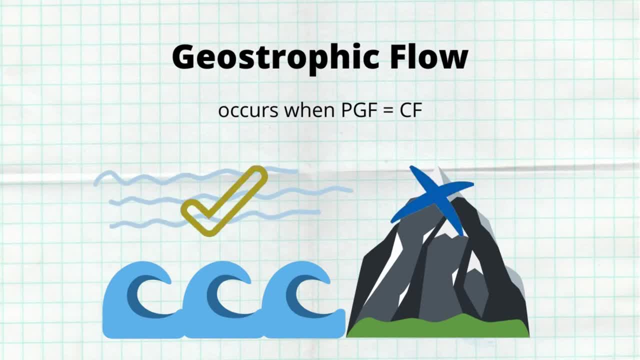 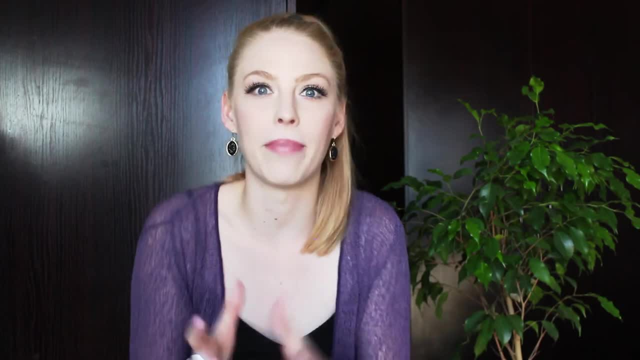 Geostrophic flow only occurs in the upper atmosphere and over oceans, where there is very, very little friction. So if we were to look at all three of these concepts on one combined, we would see that the pressure gradient force is equal to Coriolis force. 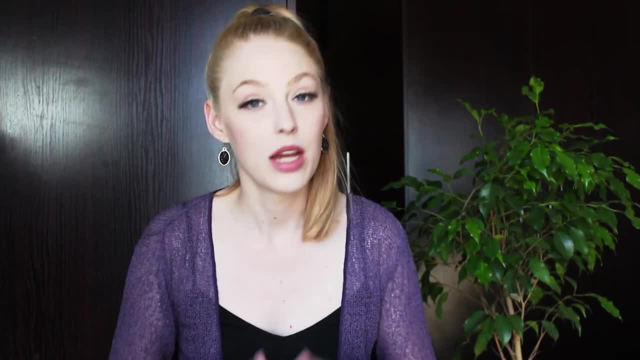 So if we were to look at all three of these concepts on one combined, we would see that the pressure gradient force is equal to Coriolis force. So this graph is just a line diagram. It would look something like this: Pressure gradient force means that air moves from a. 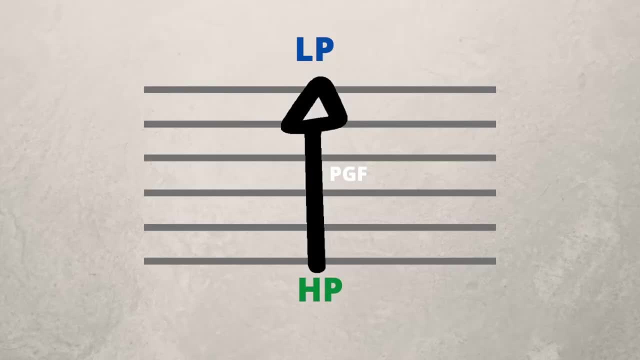 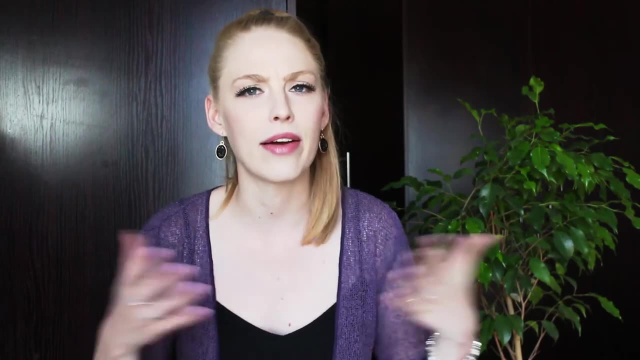 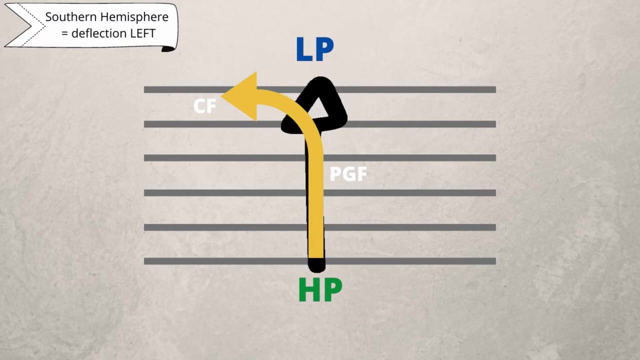 high pressure to a low pressure across the isobars. Because of earth's rotation, Coriolis force is going to cause the wind to be deflected. Now, if we are looking in the southern hemisphere, this wind will be deflected to the left If Coriolis force and pressure gradient force